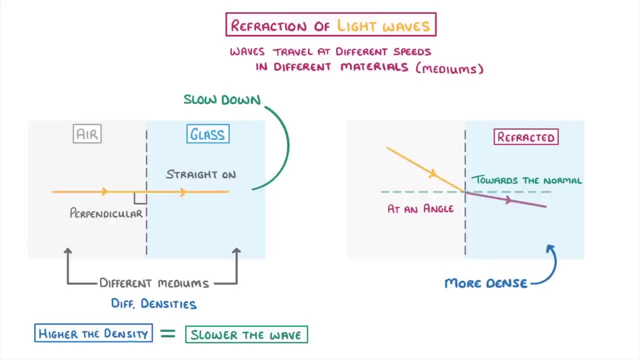 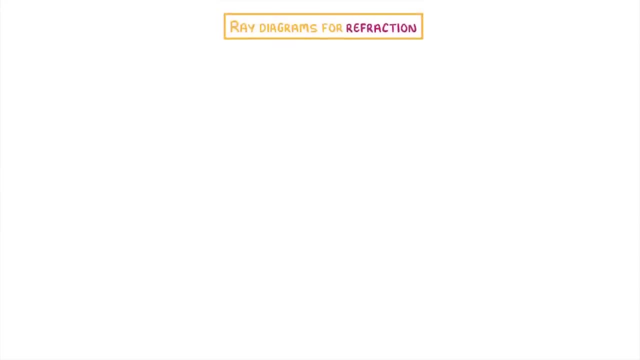 upwards a little bit towards our normal. The next thing we need to look at is how to draw proper ray diagrams for refraction. Let's imagine that we have a piece of glass with an incident or incoming light ray like this and we have to draw the full ray diagram for the transmission of the ray through the 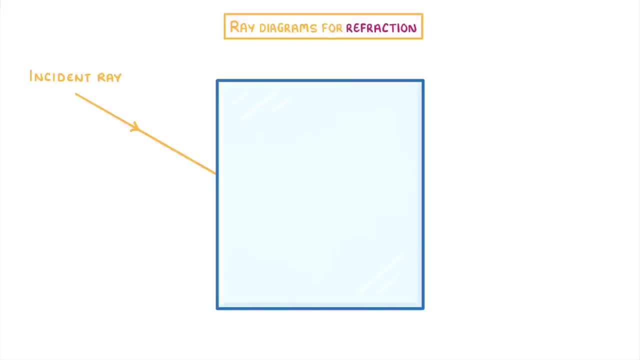 piece of glass. The first step is to draw our normal, which will be perpendicular to the glass surface, at our point of incidence, Which is where the light ray hits the glass. Now we know that if the incident ray didn't change direction, then it would look like: 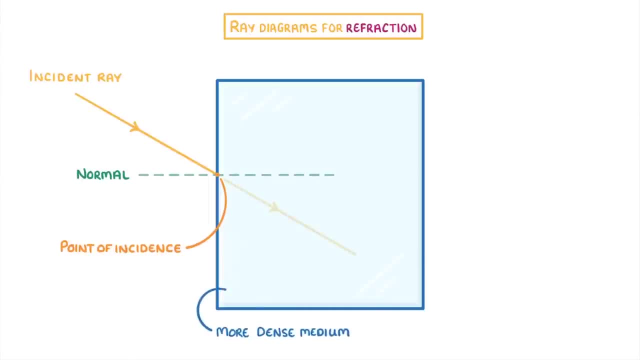 this. But because it's entering a more dense medium, the wave will slow down and bend towards the normal, So we're gonna have to draw it somewhere in this region. In your exam, it shouldn't matter exactly where you draw the new line. 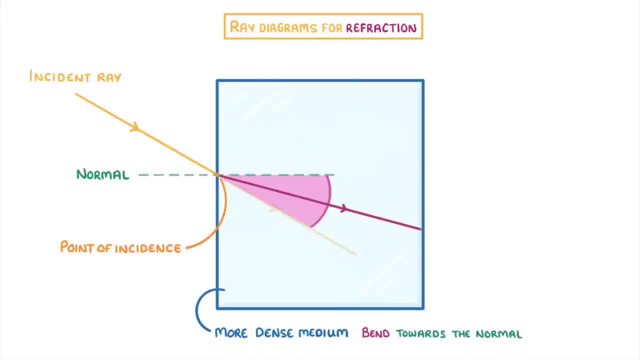 So I suggest just drawing it about halfway towards the normal, like we are here. We call this line the refracted ray and we have to continue it all the way to the other side of the piece of glass. At this point we just repeat the process. 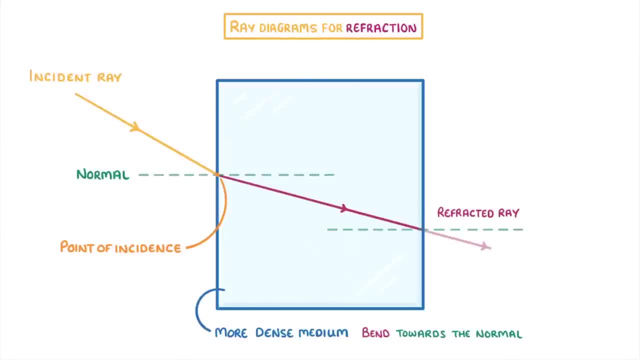 So we draw our normal, think about where the ray would be if it didn't change direction and then consider which way it's gonna bend. This time it's passing from the more dense glass to the less dense air, So it will speed up and bend away from the normal. 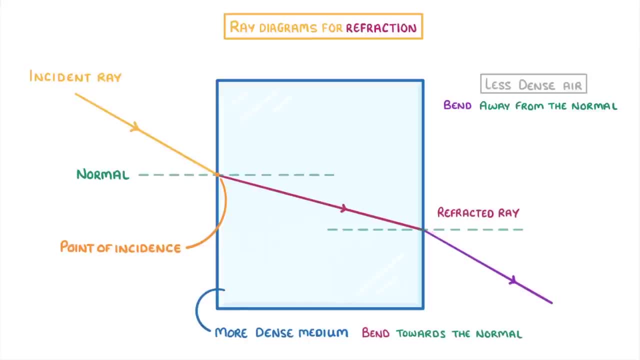 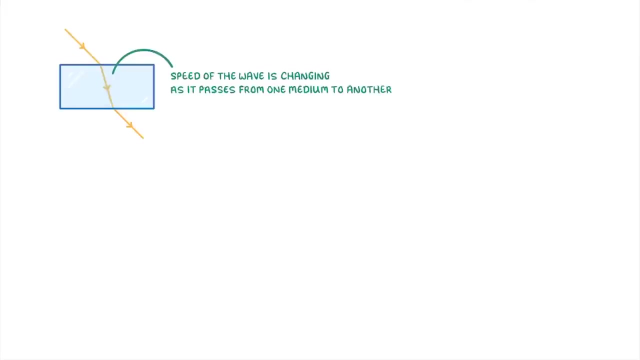 So something like this, And we call this ray the emergent ray. To complete the diagram, we also need to add the angle of incidence and the angle of refraction as well. The last thing I want to mention is that, because the speed of the wave is changing,